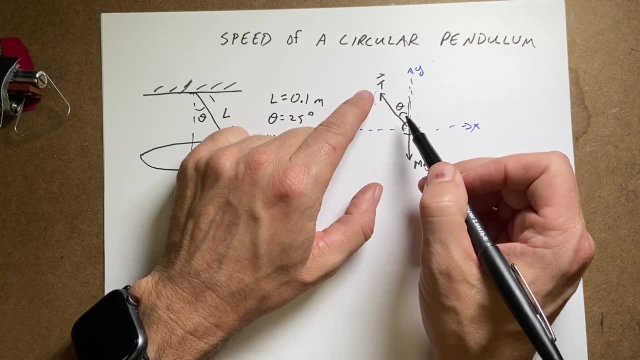 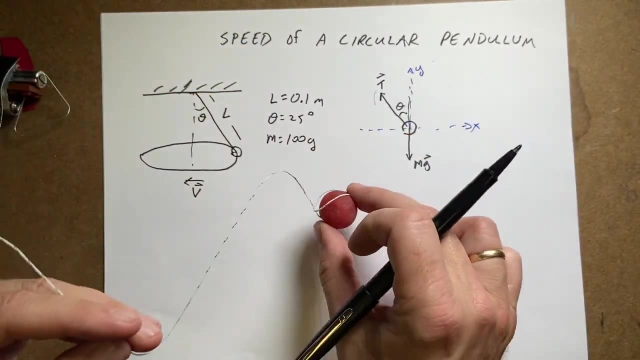 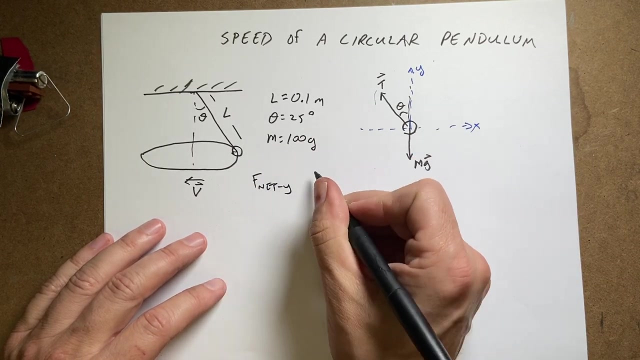 the tension formula. But what I can say is that I know the direction of the tension force and I know something about the motion of this ball, Because as this thing moves around in a circle like this, its vertical acceleration is zero. So I can write f net in the y direction, just the y. 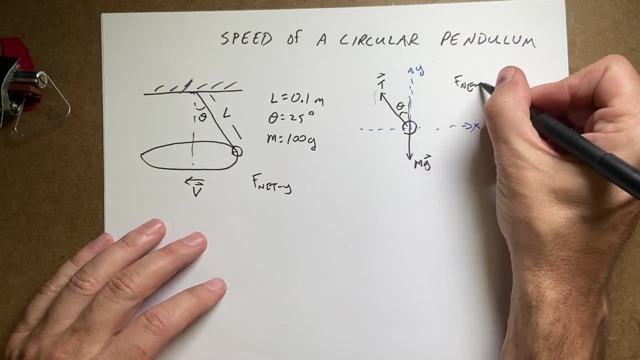 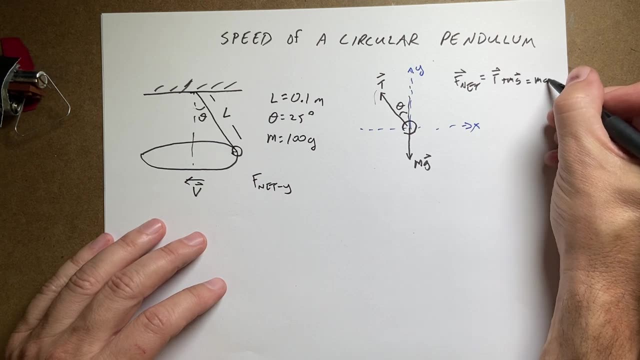 component. If I wanted to write f net it'd be like this: f net equals t, plus mg equals ma As vectors. But that's not very useful. If I break it into the x and y direction I can say the net. 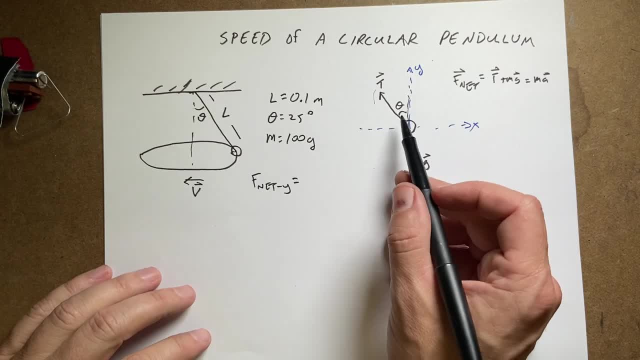 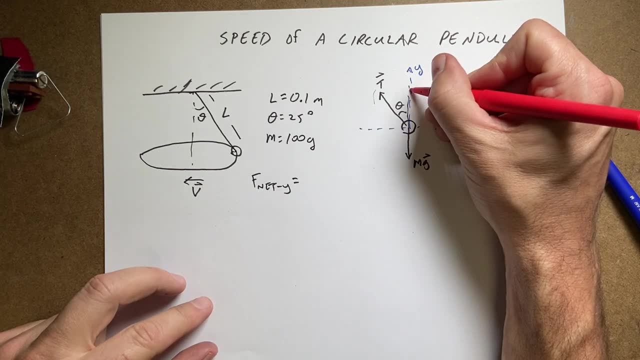 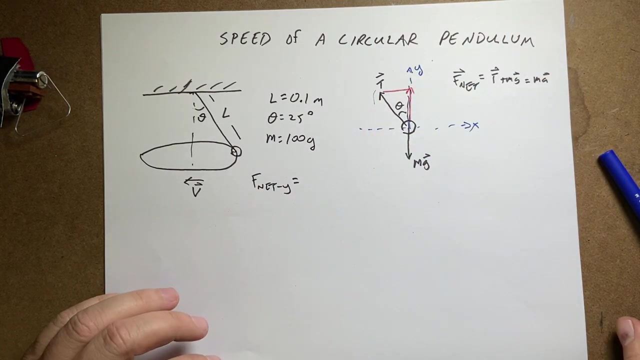 force in the y direction has to be zero, right, Because it's not accelerating. So what forces are in the y direction? Well, I have, my red marker is dying. I should have gotten a new one. So here is the y component of the tension, Here is the x component of the tension. So this whole length. 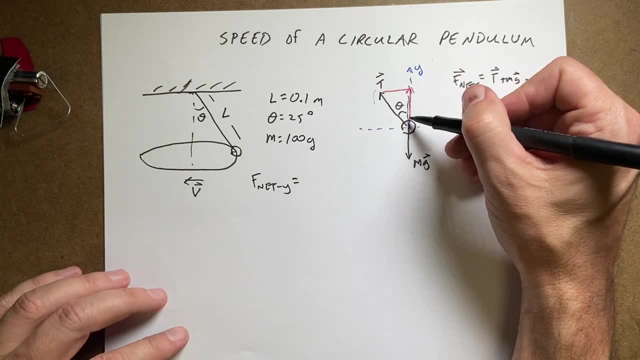 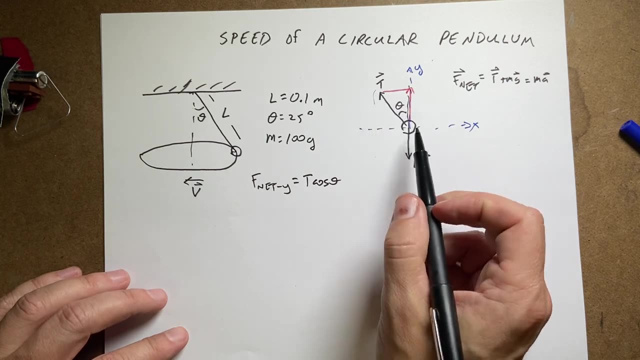 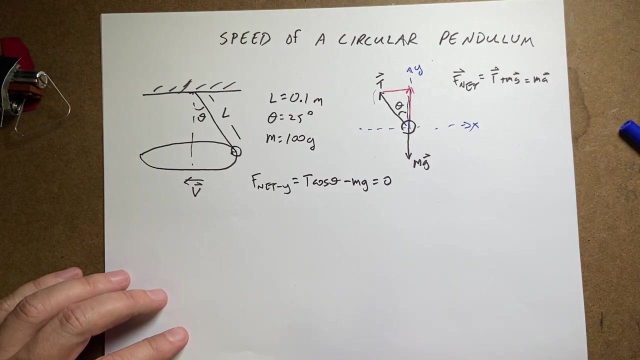 is t the tension And this is the adjacent side. So this is going to be t cosine. theta is the y component of that tension. What's the y component of the gravitational force? It's going to be minus mg And that equals zero. So in this case I actually know theta is 25. 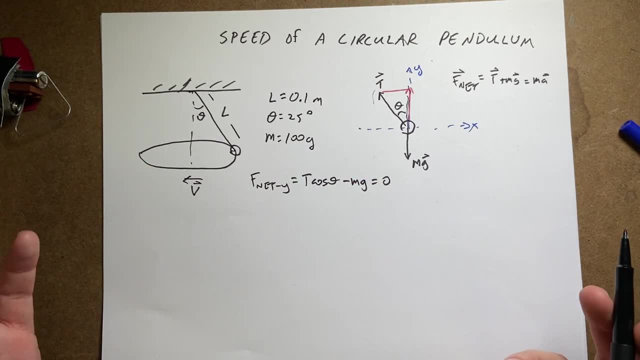 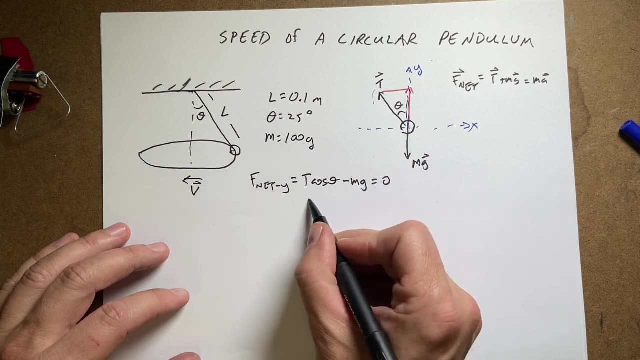 degrees. I picked that. I know m, I know g, So I'm pretty good right here. Let's go ahead and solve this for tension. That's the only thing I don't know. So if I add mg to both sides, I get. 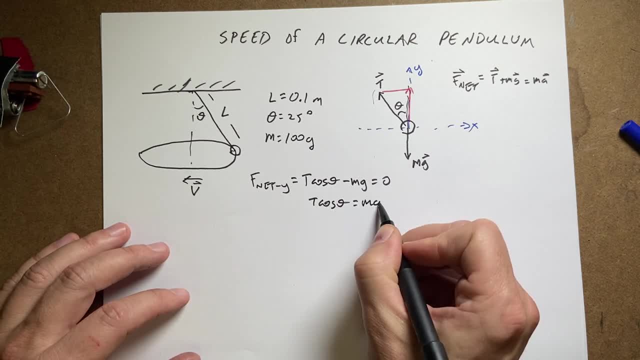 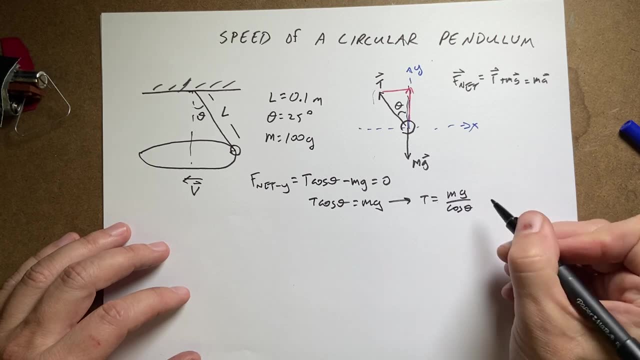 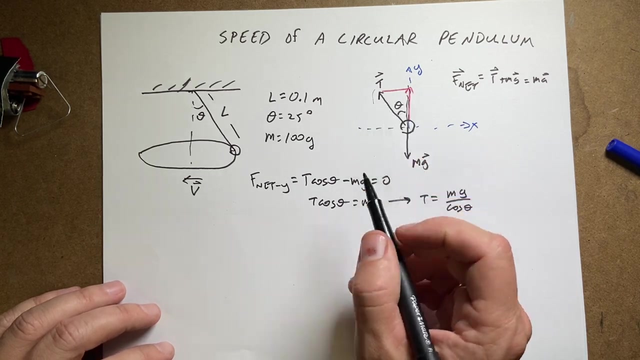 t cosine theta equals mg. And then I can solve for t: t equals mg divided by cosine theta, which, so I know everything there. Now let's look at the y direction, I mean the x direction. So in the x direction, what forces are there? I can say f? net. 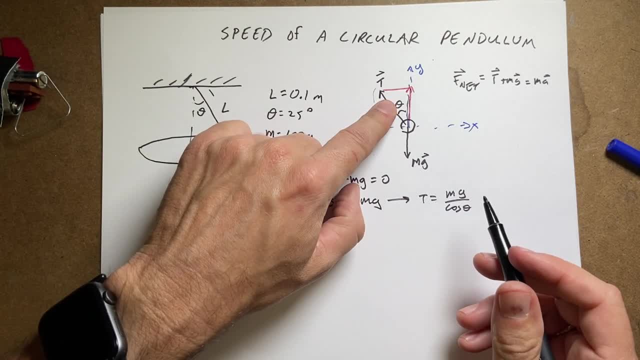 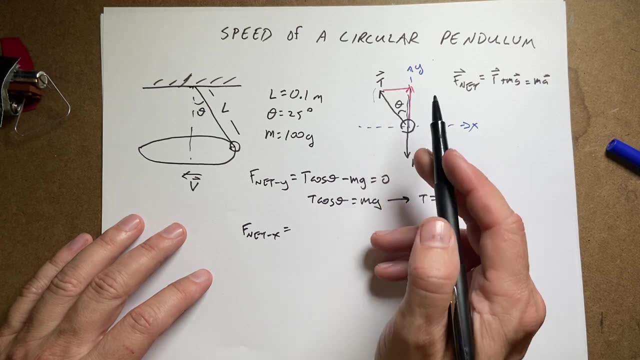 x equals there's only one force that has component in the x direction, and that's t. So the opposite side of this triangle is the x component of the tension. So that's going to be sine of theta, So it's going to be minus t. 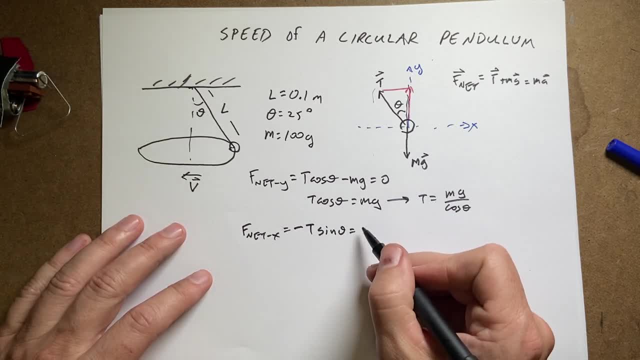 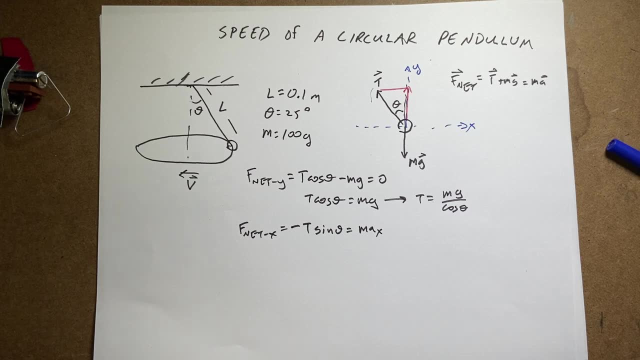 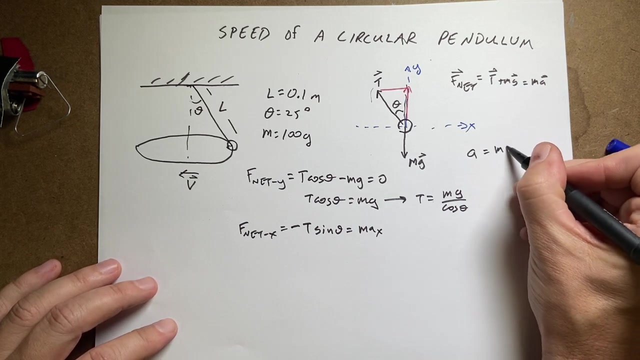 sine theta, And that's going to be equal to m, a, x. So here's something we know about a circle. If it's moving in a circle at a constant speed, then a is going to be equal to m, v squared over r. 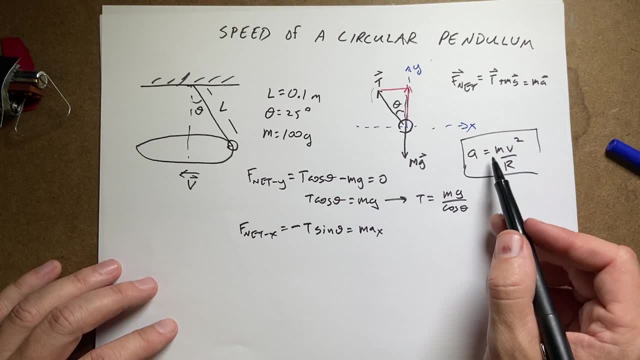 That's the acceleration pointing in the magnitude of the acceleration and the direction. it's pointing towards the center of the circle. So in this case it's accelerating that way, in the same direction as that component. So that's going to be equal to m a x. So that's going to be. 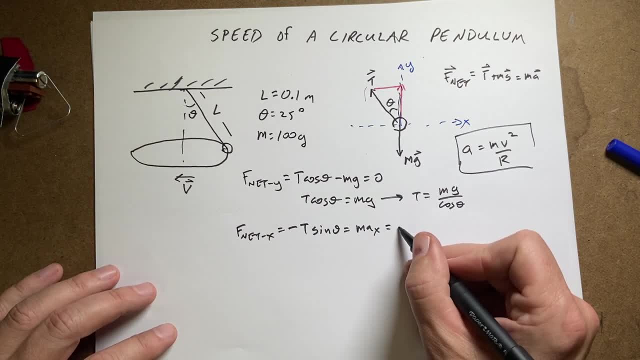 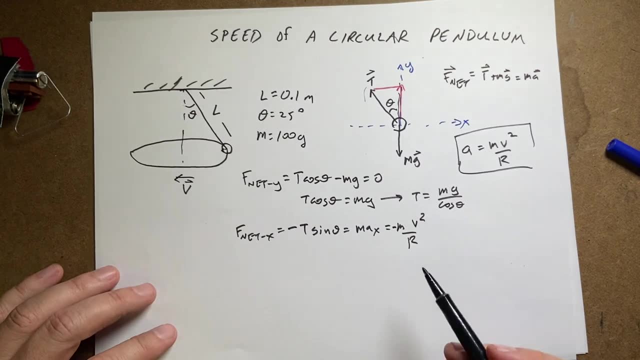 equal to m a x. So that's going to be equal to m negative v squared over r. So it's in the negative x direction. The negatives cancel. I'm trying to solve for v, so let's just solve this for v: The. 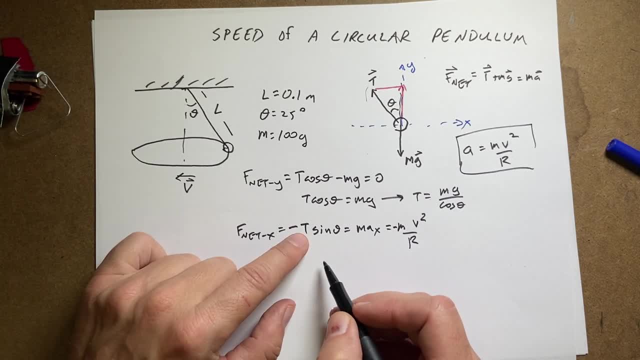 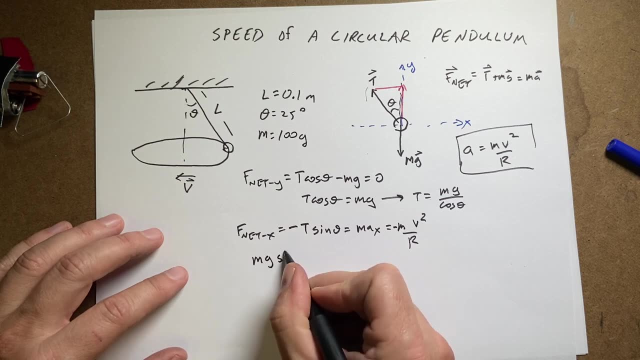 mass cancels. No, the mass it does, it's going to cancel. So I'm going to put in my value the negative signs cancel. I'm going to put in my value for t, So I get mg sine theta over cosine theta. 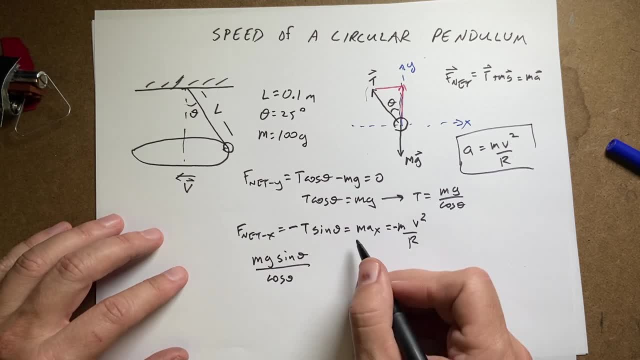 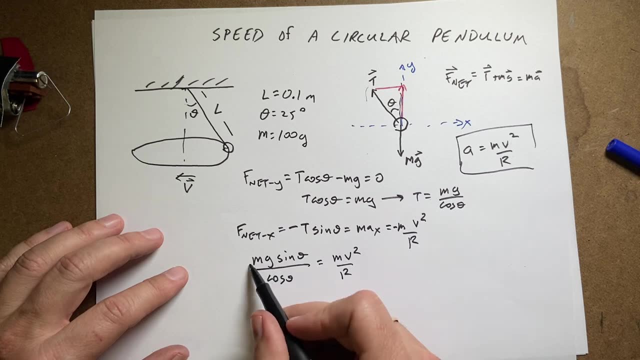 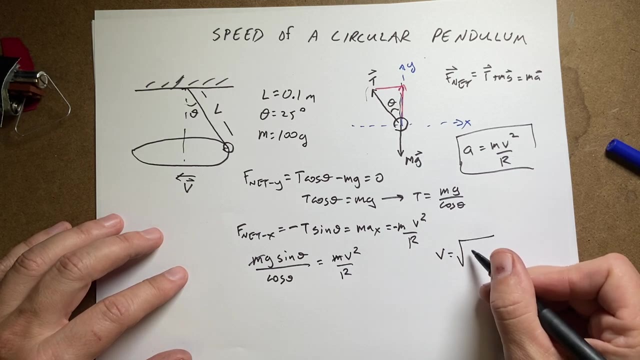 that's t, that's sine theta. so that's what I get: equals mv squared over r. Now I can solve for these masses: cancel and I can multiply by r and take the square root and I get v equals the square root of rg. 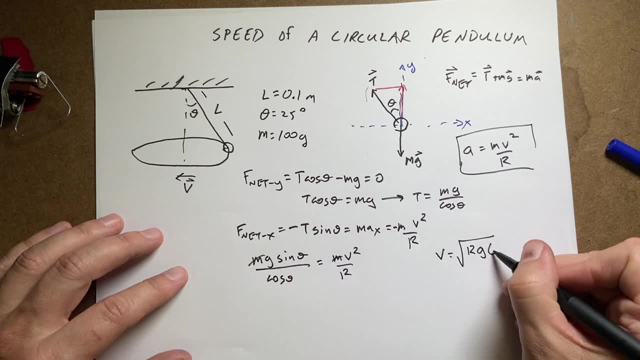 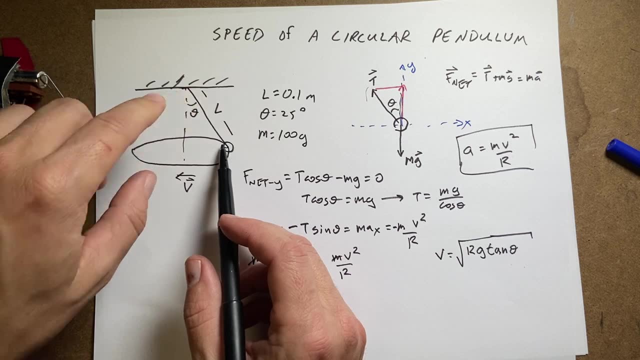 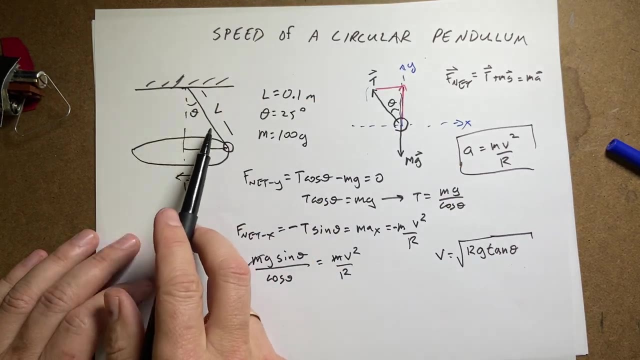 and I have sine theta over cosine theta is tangent theta, Okay, but I don't. I know the length of this is 0.1 meters, but I don't know this r, but I can find it right Because now I look at this triangle, here's 0.1 meter long. 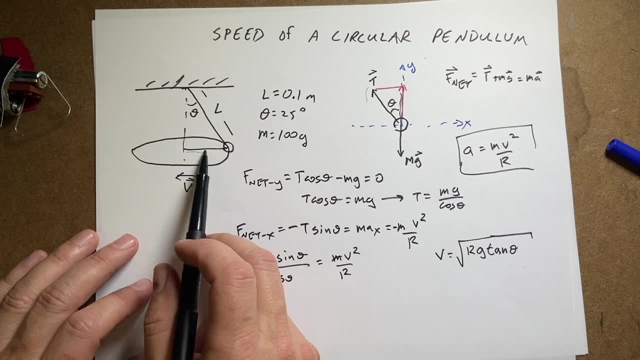 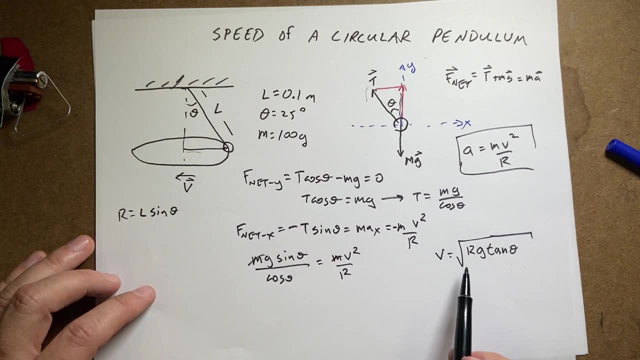 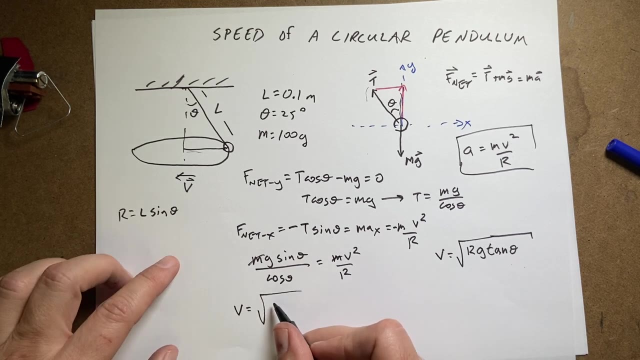 the angle is 25 degree theta, so this would be l sine theta, So r equals l sine theta. So I can put that in over here. actually, let's put that back as tangent, so I get v equals equals the square root of r. 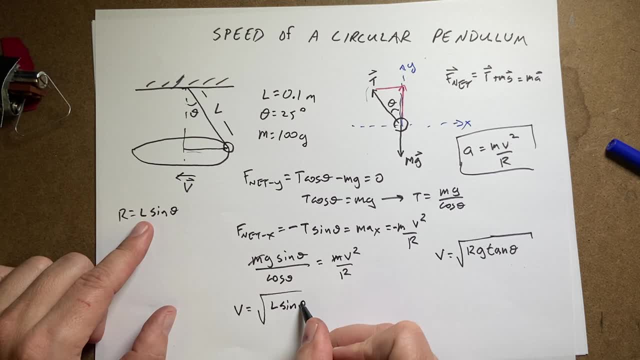 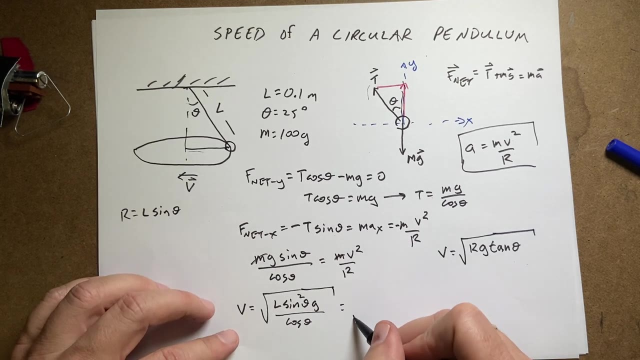 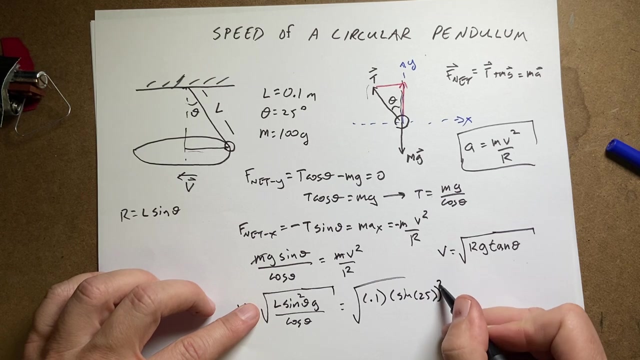 which is l sine theta times g times sine theta. so I have sine squared theta over cosine theta. Okay, let's put in our values. so I'm going to get square root of 0.1 sine of 25 degrees squared. 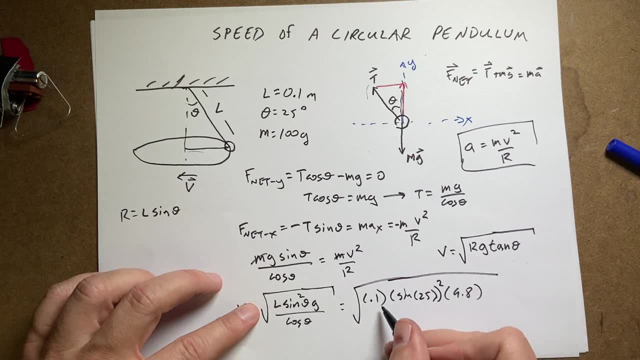 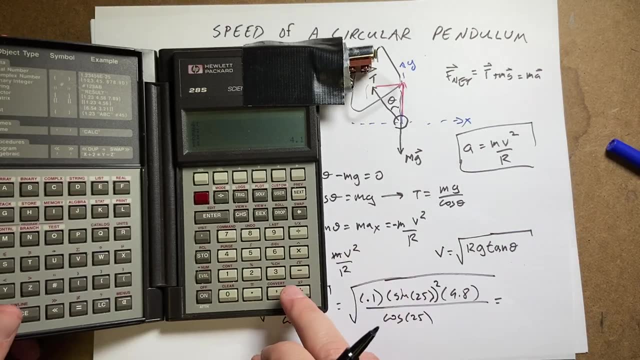 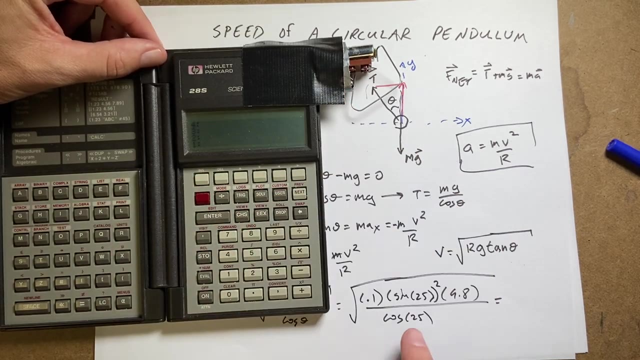 9.8, divided by cosine of 25.. And let's put that in the old calculator. Okay, so again I'm using my RPN Hewlett Packard 28S. I know you're jealous with the custom battery pack.